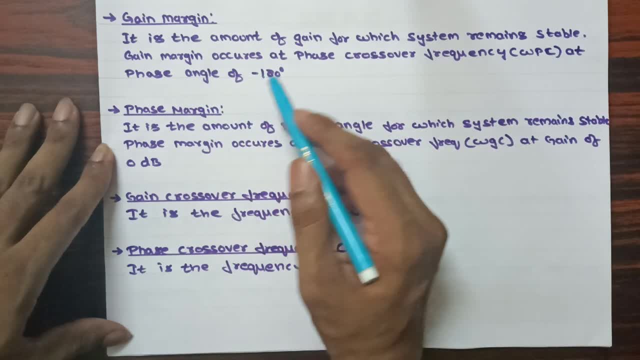 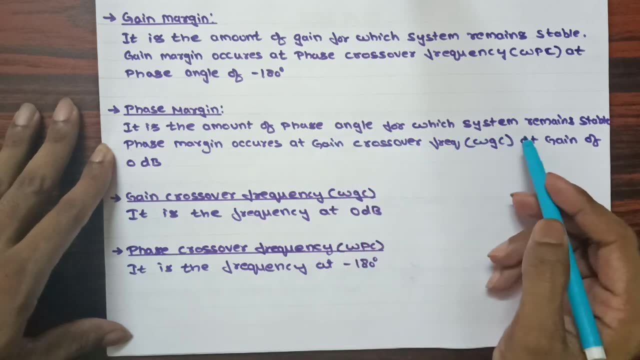 of minus 180 degree. Gain margin is: it is the amount of gain where the system remains stable. Phase margin: it is the amount of phase angle for which system remains stable. Phase margin occurs at gain cross over and denoted by omega gc at gain of 0 dB. 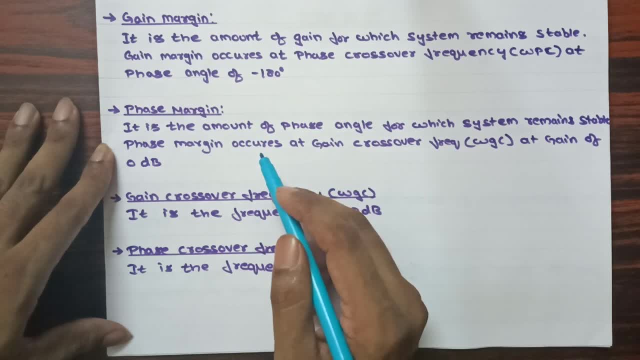 So in this also it is an amount of phase for which the system remains stable and it occurs at gain cross over frequency, that is, at gain of 0 dB. Gain cross over frequency: It is the frequency at 0 dB. and phase cross over frequency: it is the frequency at minus. 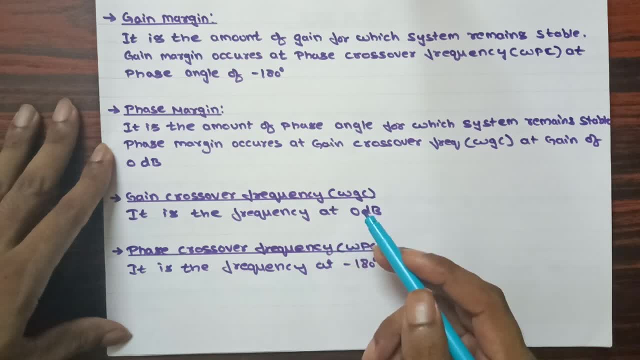 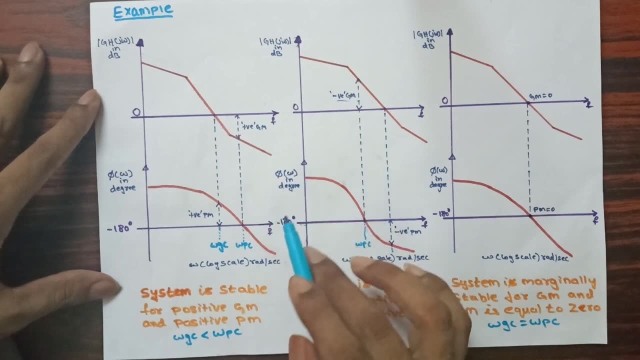 180 degree. So this will understand better from the Bode plot. In this you can see that I have considered Bode plot example for three conditions. that is, one plot is for stable system and the second plot is for unstable system and the third plot is for marginally stable system. 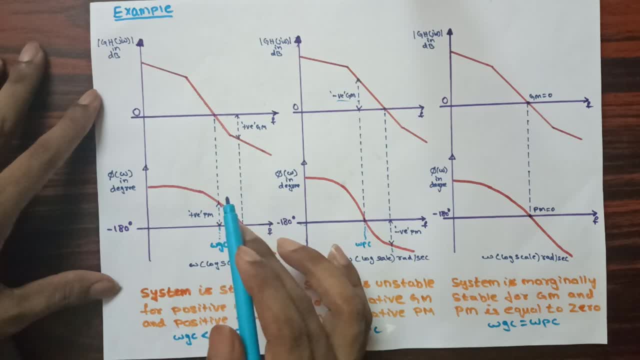 In this plot. As I said, Bode plot has two parts, that is, magnitude plot and phase plot. You can see that this is the magnitude plot and this is the phase plot. In this x axis we have considered log scale, that is, omega log scale. radians per second. 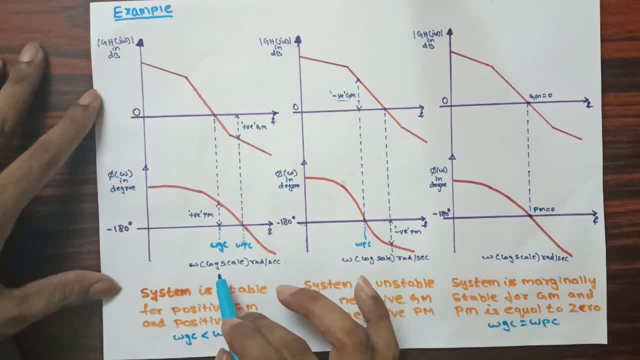 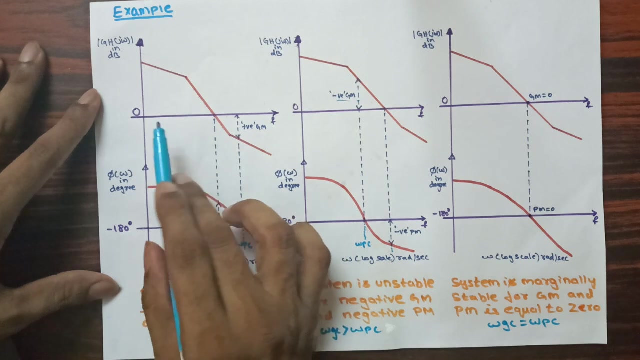 The frequency where the log scale we have considered and the log scale will be available in semi log sheet. So here you can see that for phase plot we have considered in the y axis, phi of omega in degree And the reference line. you can see that for phase plot we have considered minus 180 degree. 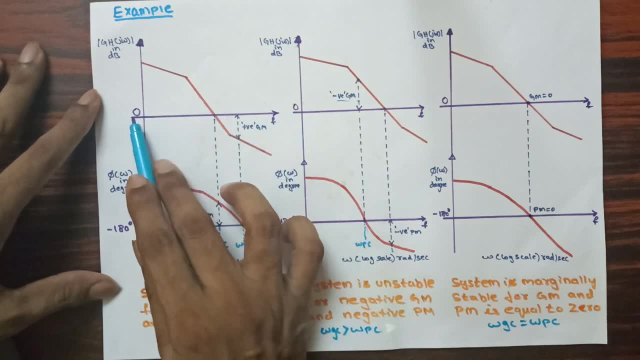 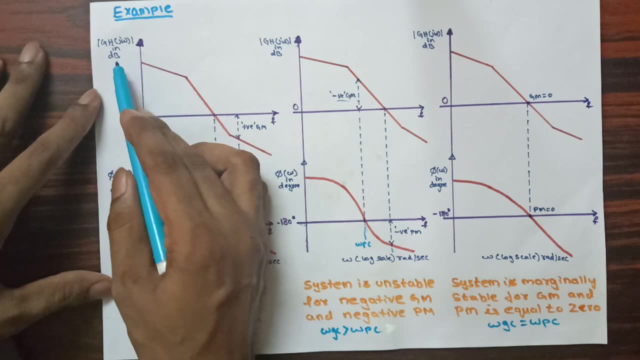 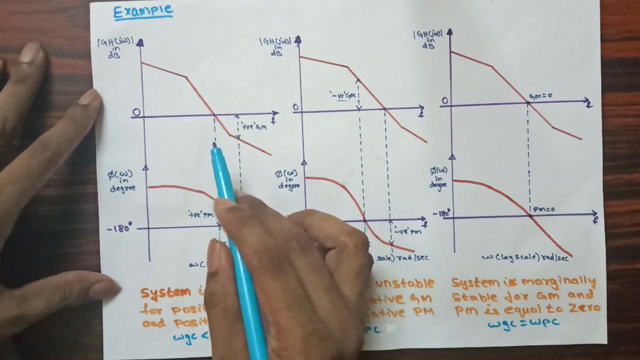 And in the magnitude plot, the reference line, you can see that we have considered zero axis here and in y axis we have considered the magnitude of gh, of j, omega in dB. So now in this we are going to measure the phase margin and gain margin to measure the. 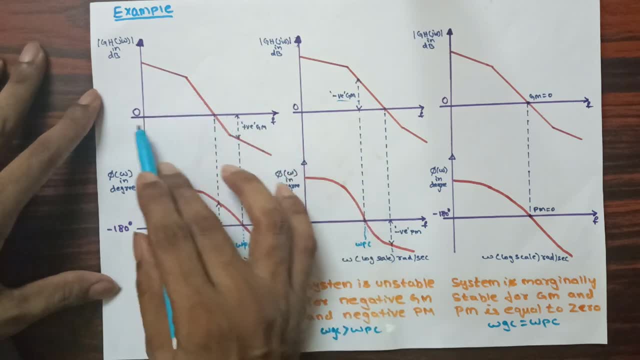 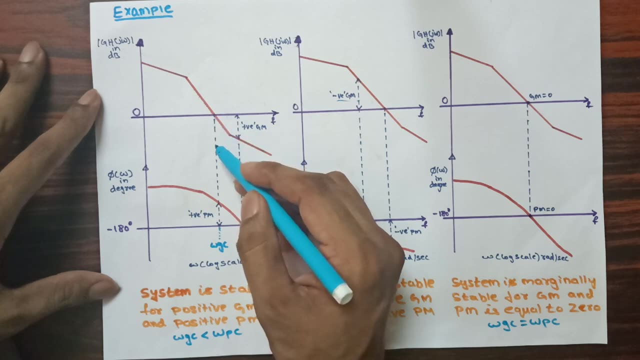 phase margin. We are going to see the magnitude plot crossing the zero axis. So here you can see that the plot is crossing At this point. So from this point we are going to extend till down, which is going to be considered as a gain: crossover frequency. 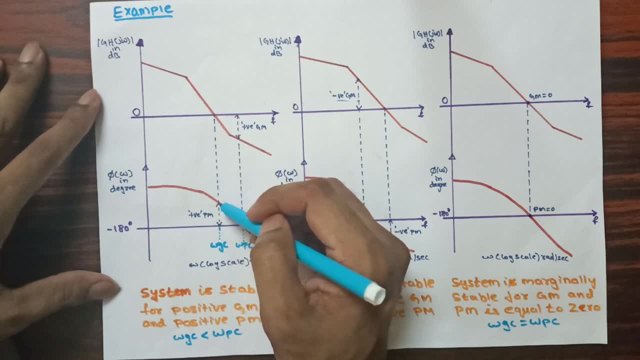 Now, at the same view, you can see that it is stretching to the plot, that is, to the phase plot. from the point where it is stretching to the phase plot, to the reference line, that is minus 180 degree, We are going to measure the phase margin. that is a positive phase margin. 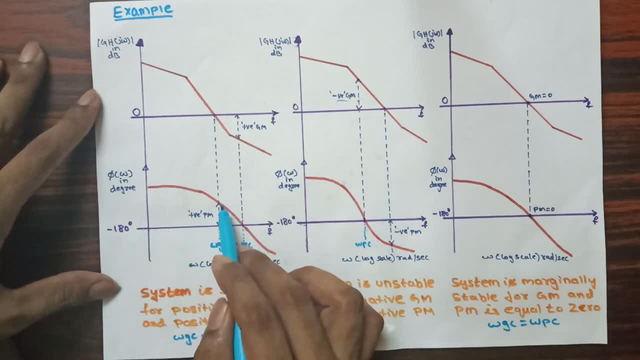 If you are getting a value above the minus 180 degree, then it is a positive phase margin Next, So to calculate the gain margin, we are going to consider the phase plot. You can see here the phase plot is crossing to the minus 180 degree to measure the gain. 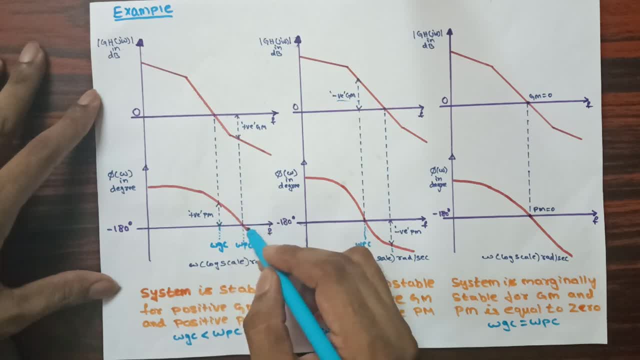 margin. We are going to consider the plot crossing the minus 180 degree and will extend down to get the phase crossover frequency and to get the gain margin. We are going to extend above till it touches to the magnitude plot. The point where it touches to the magnitude plot, to the zero reference line, we are going 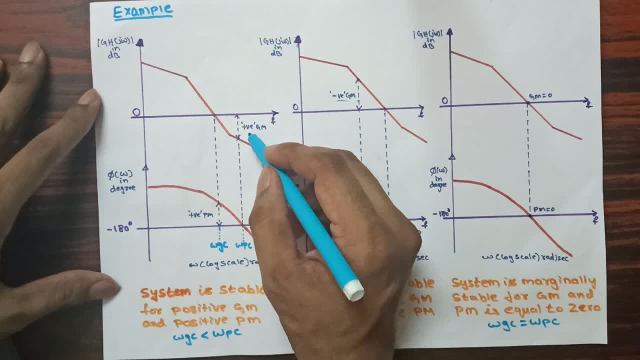 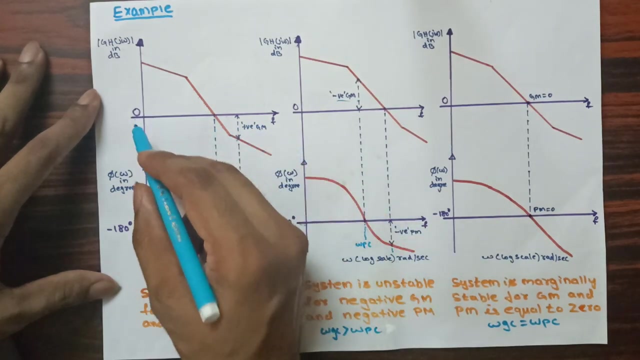 to measure the value And that value, whatever we get, that is the positive gain margin In this, remember, below zero axis is a positive gain margin. If you get any value above zero axis then it is a negative gain margin And in this first example, I am getting the gain margin below the zero axis. 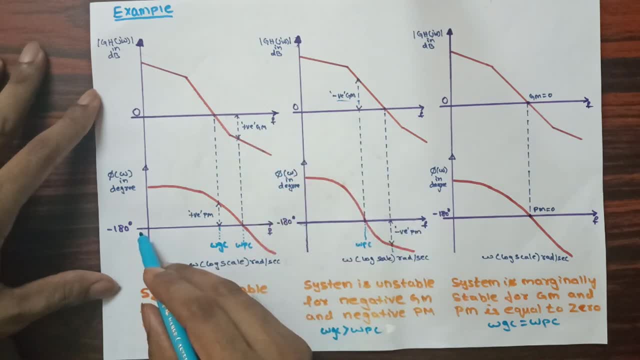 Therefore it is a positive gain margin And in this I am getting the phase margin above minus 180 degree. that is positive phase margin. Both are positive. Therefore system is stable. Remember to get the positive gain margin. we are going to get the phase margin above. 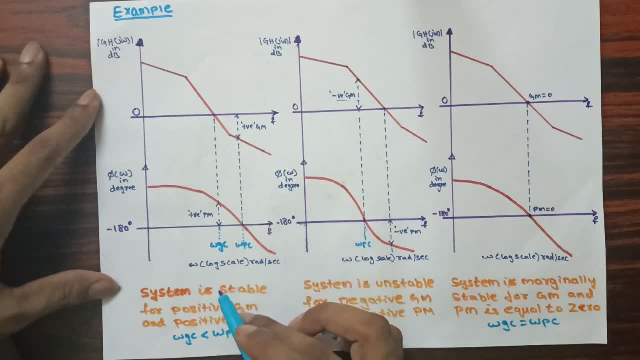 minus 180 degree. And in this second example we are going to check the stability: The phase margin and gain margin. both should be positive. If any one also becomes negative, then the system is unstable. So in this way we are going to comment on the stability. 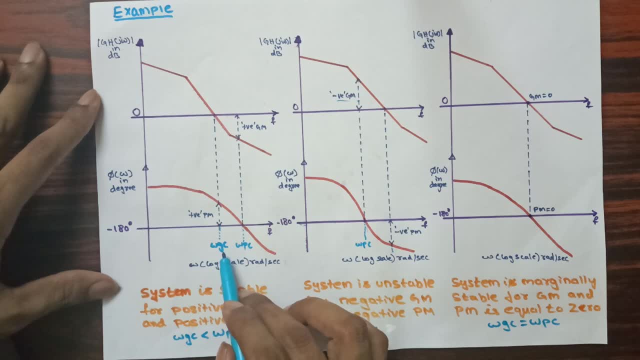 And also you can see here the gain crossover frequency is lesser than the phase crossover frequency For a stable system. this also you can remember: the gain crossover frequency is lesser than the phase crossover frequency. Next, in the second example, how to consider for the unstable system, 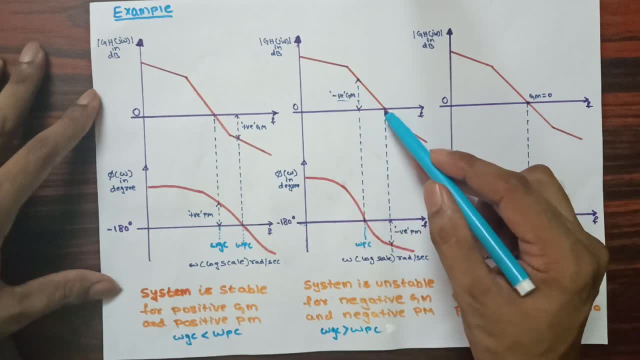 here you can see that the plot crossing at zero axis. from that point i'm going to measure the omega. from this point i'm going to measure the gain crossover frequency by extending till down and at the same time i will see that when the point it touches to the plot, from that point to 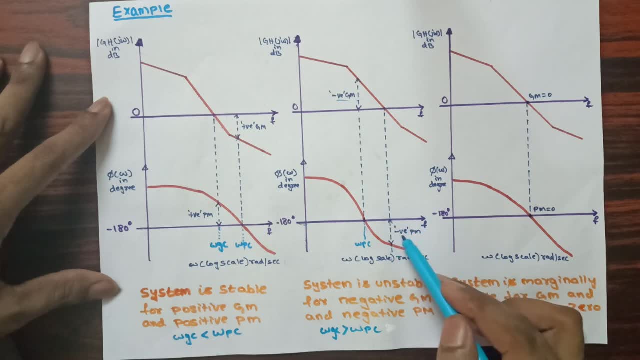 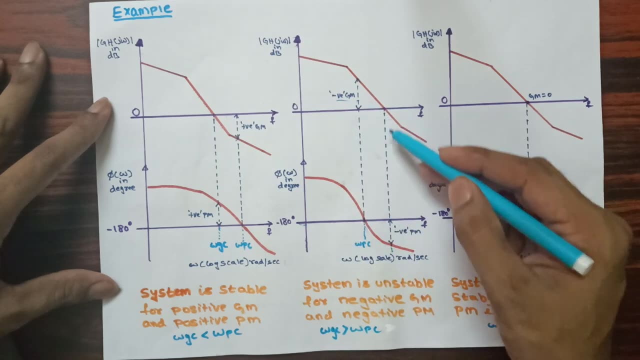 the reference that is minus 180. i'm going to measure the phase margin here. in this case. you can see that at the plot, the magnitude plot, where it crossing to zero axis, have extended down and you can see here this point, have touched to the plot from that point to the reference point i. 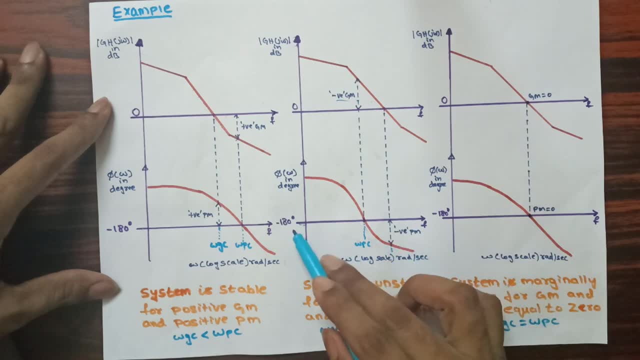 have considered the phase margin, but this value i'm getting below minus 180 degree. therefore it is a negative phase margin. so, whereas for gain margin calculation, we are going to look into the phase crossover, that is, at the point where the plot crossing to the minus 180 degree, we are. 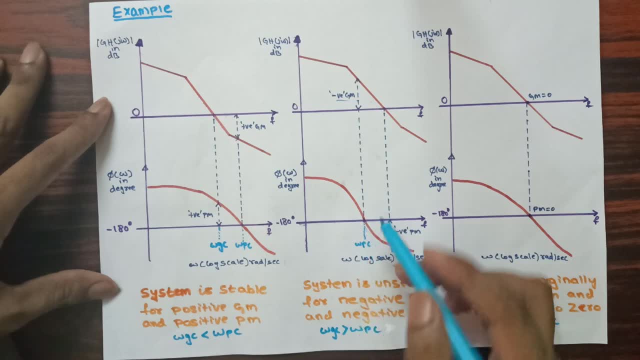 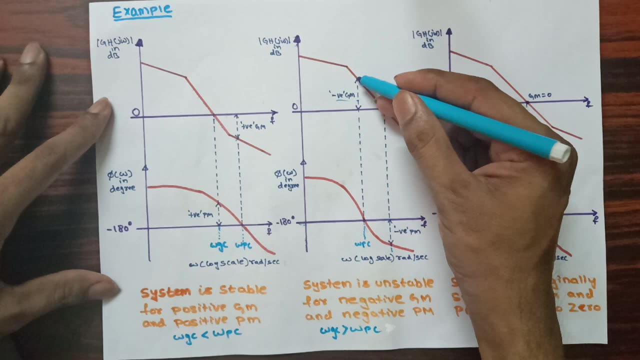 going to get the phase crossover frequency. if you extend down and if you extend up then we are going to get the gain margin. so we are going to extend till it touches to the plot from the point where it touched, from that point to the reference- zero reference. we are going to measure the value that. 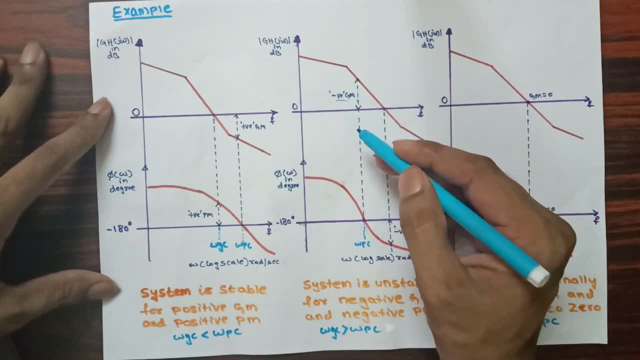 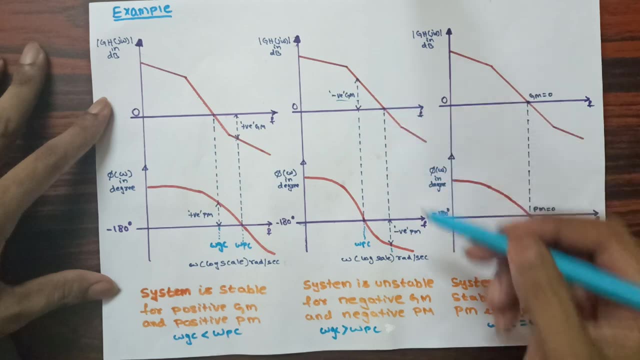 is considered as a gain margin. here you can see the value i'm getting above the zero axis. therefore it is a negative gain margin. in this example, i am getting here negative gain margin and negative phase margin. therefore it is a unstable system. and also you can see here phase crossover frequency. 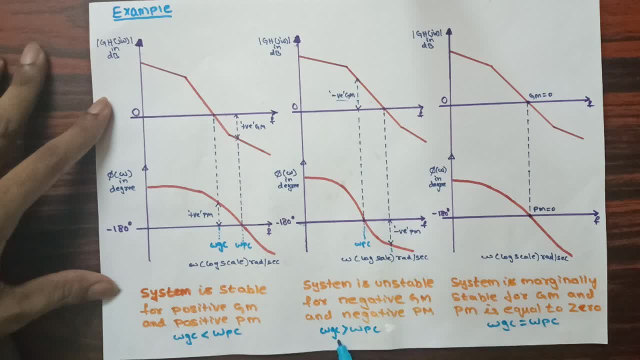 is lesser than gain. stop. Ok, we have considered only 0 at the point when the phase hours take %. Now we are gonna see this length reaching a cross over frequency. Omega gc is greater than omega PC for unstable system, so next in we considered the third example for marginally stable system. for that. 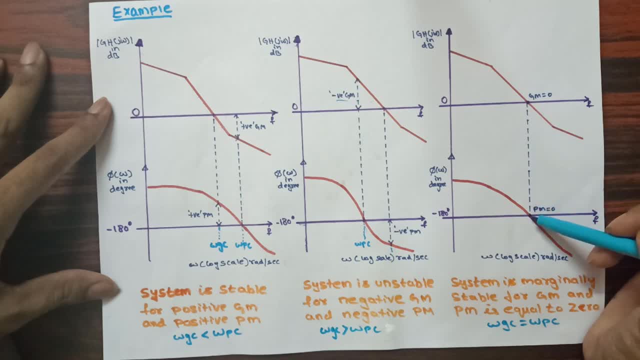 you can see here the magnitude plot crossing at zero axis. when we extend this point up below, then you can see here it is exactly, it is coming to the mind of the plot- phase plot crossing at a minus 180. so here. So at a 0 crossing of magnitude i am getting, phase margin is equal to this point. 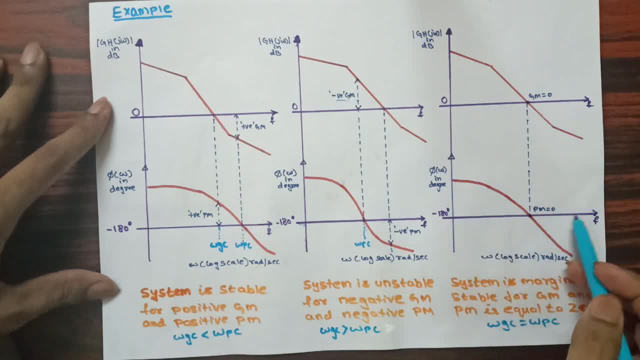 So that means i have to consider the space fiction at this point, Learning the value that each and every point take. at lower velocity talladeunden we more than andney 0 and phase plot crossing at minus 180 I am getting. if I extend above, I am getting gain. 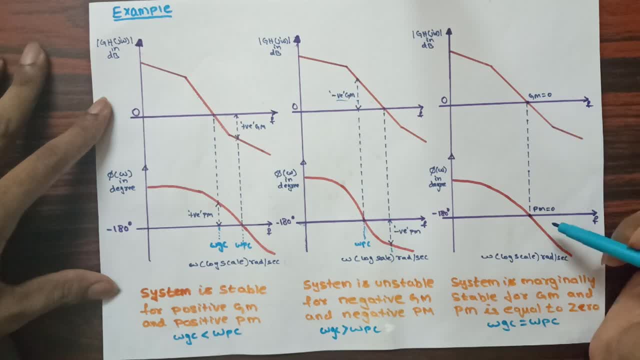 margin is equal to 0. So in this case, both gain margin and phase margin is equivalent to 0. therefore, the system is marginally stable. In this way we are finding the stability of the system. These are the three examples I have taken in Bode plot to explain the stability of the 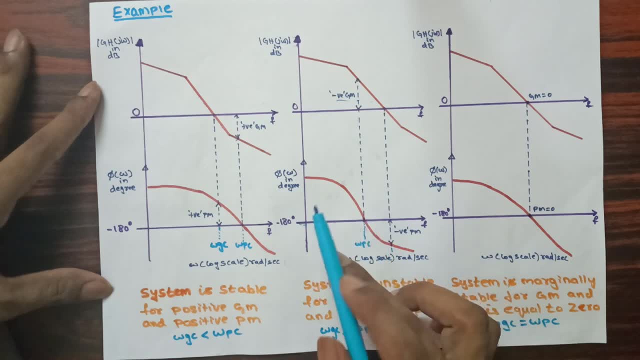 system. So, depending upon the problem, I may get positive gain margin or negative gain margin, or negative gain margin or positive gain margin, as here in these three cases we saw. both are positive, stable, both are negative, unstable, So both are equivalent to 0, marginally stable, Remember any? 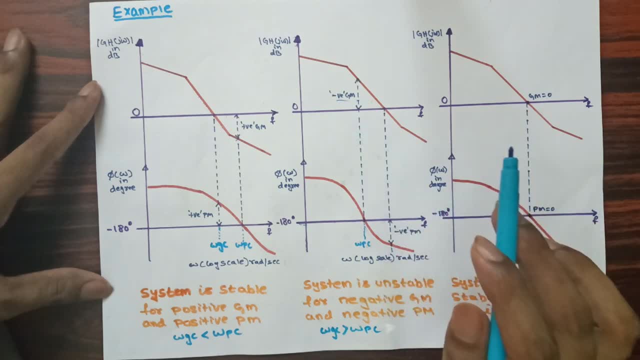 one also negative in the plot gain margin or phase margin, then the system is unstable. and if you are getting the response, suppose, in the problem, if the response is not crossing to the minus 180 degree, then the gain margin will be 0. infinite. If I get the positive phase margin and the gain margin is infinity, then the system is. 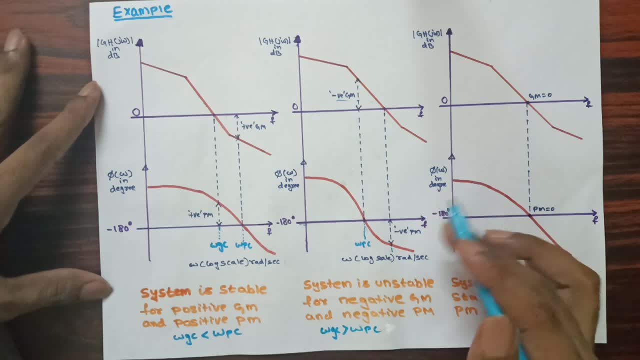 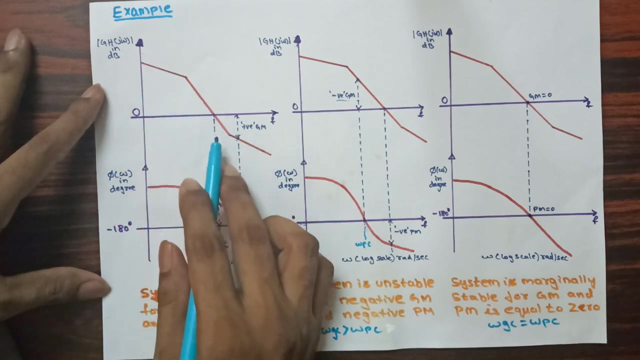 stable. So these are some examples when we so these are some examples to be remember when we solve the problem. Next video we are going to discuss initial gain, that is to start the graph, and then we are going to see the initial slope and change in slope, that is, in the magnitude plot. 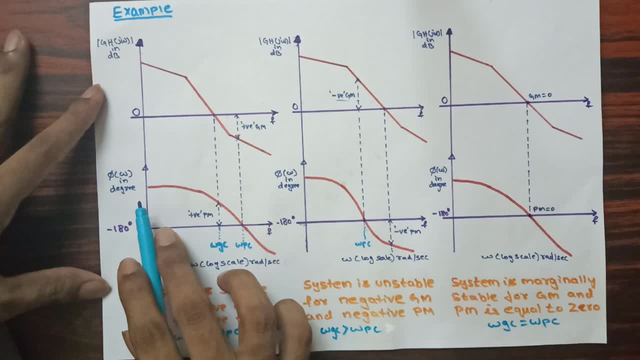 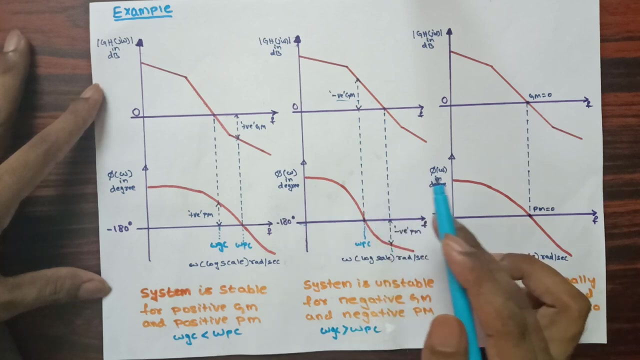 table and we are going to see the formula that is to get the phase angle values. So how to form the phase angle formula that also will we are going to discuss in the next video. Hope you understood this video. for more such videos, like and subscribe my channel. Thank you. 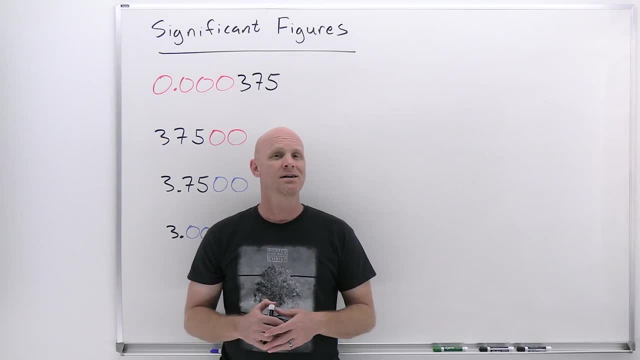 Significant figures and scientific notation are going to be the topic of this lesson, So we're going to do a lot of calculations in this course and knowing how many digits to include in an answer. So, as well as being able to write really little numbers and really big numbers, 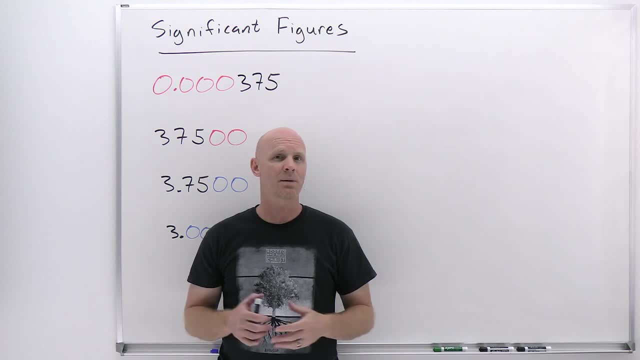 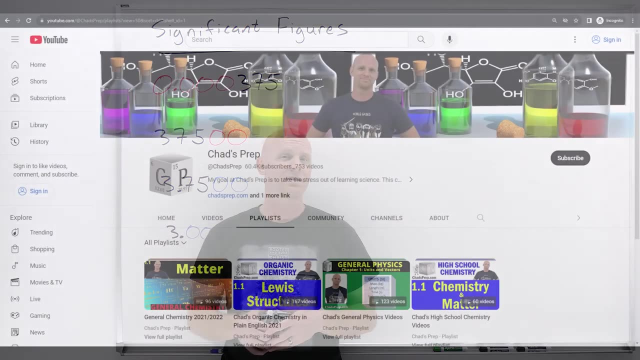 in scientific notation is going to prove important. Those are the two topics in this lesson. My name is Chad, and welcome to Chad's Prep, where my goal is to take the stress out of learning science. Now, if you're new to the channel, we've got comprehensive playlists for general chemistry. 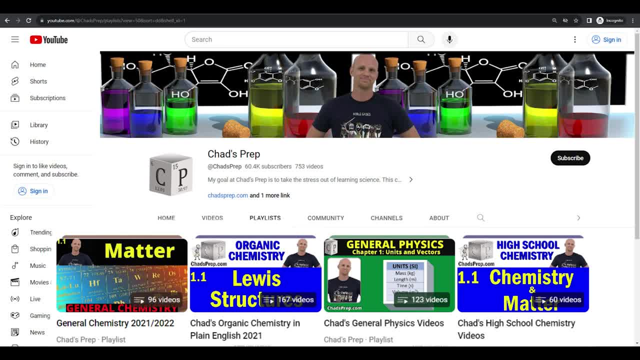 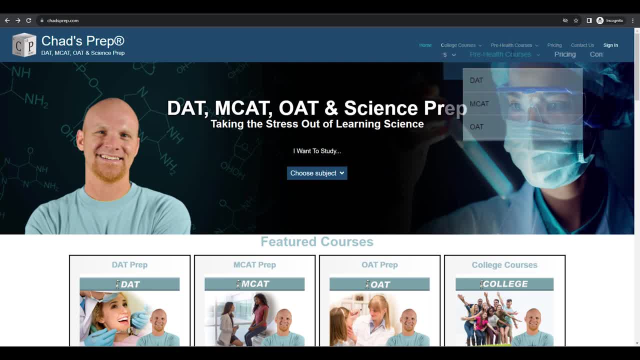 organic chemistry, general physics and high school chemistry, And on chadsprepcom you'll find premium master courses for the same that include study guides and a ton of practice. You'll also find comprehensive prep courses for the DAT, the MCAT and the OAT.